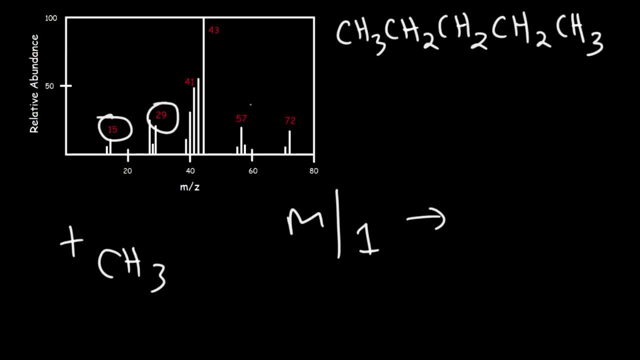 and which of these numbers these fragments correspond to. If you understand this, then you could use this to identify which molecule corresponds to which graph. But for now, let's identify the fragments that form in pentane if we put it in a mass spectrometer. So let's call this carbon 1, 2, 3, 4, 5.. Now if we break the C1C2, 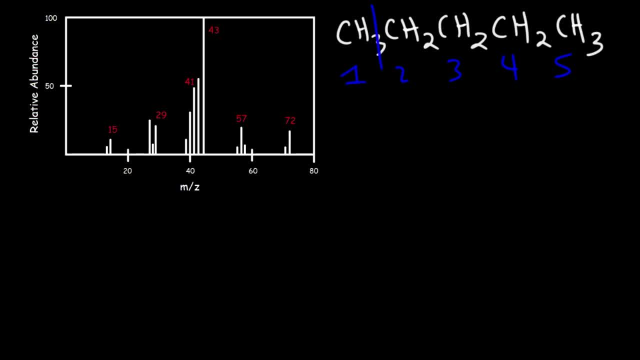 bond. it can split up into two, A CH3 group and a butyl group. Now, typically one is going to be a radical and the other one is going to have a positive charge. Now carbon has an atomic weight of 12, and hydrogen is about 1. So CH3 is 15, CH2. 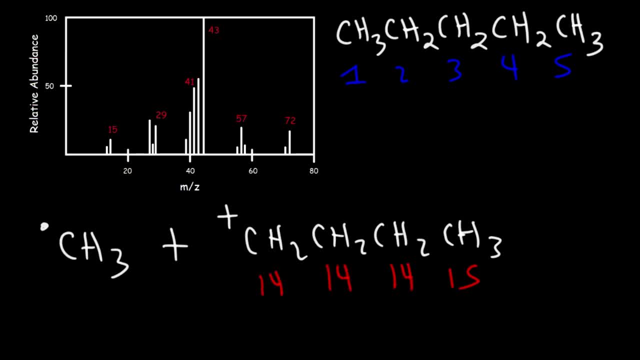 has an atomic weight of 14, and if we add up 14 plus 14 plus 15, plus another 14, this will give us 57. So 57 could correspond to this particular fragment. Now we don't always have to get a methyl radical. We could get a methyl cation If 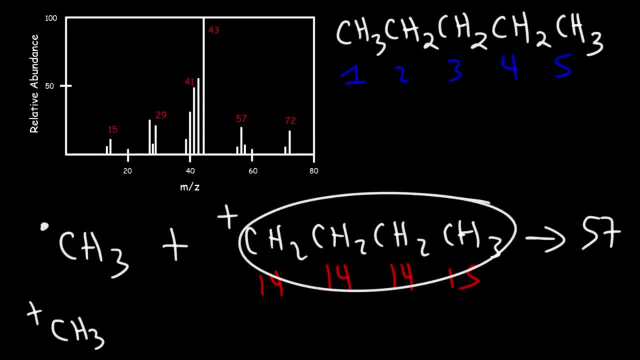 we do get a methyl cation, then this molecule will be a radical, So this is another possibility. But it's important to understand that only the positively charged fragments will reach the detector, And so the methyl cation could easily correspond to the peak that we 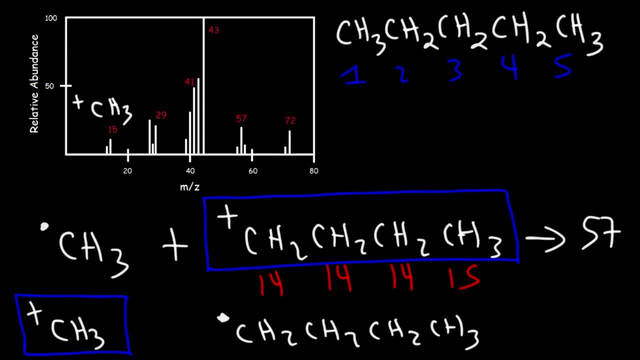 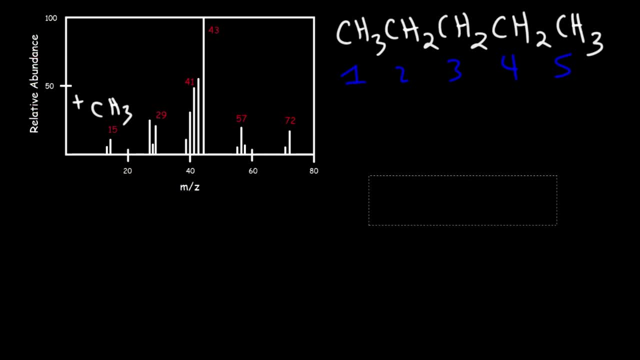 see at 15.. Now, what about the peak at 43? That peak is known as the base peak. It has a relative abundance of 100%. So everything is compared to the base peak. The peak at 72 is known as the parent peak, also called the m plus peak, And it 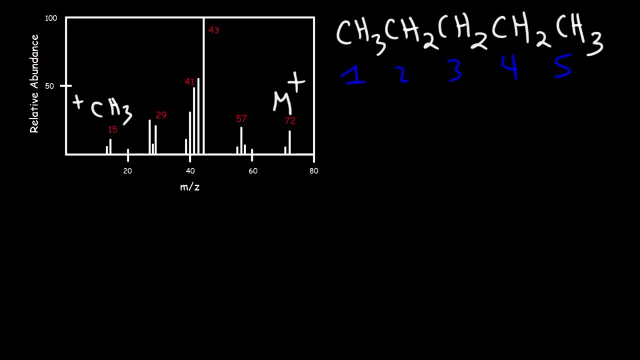 turns out that it's simply the mass of the compound. If you add up 15 and 14, 14, 14 and 15, this will give you the total molecular weight of pentane, which is about 72 grams per mole, and so that corresponds to the M plus peak. now, if we 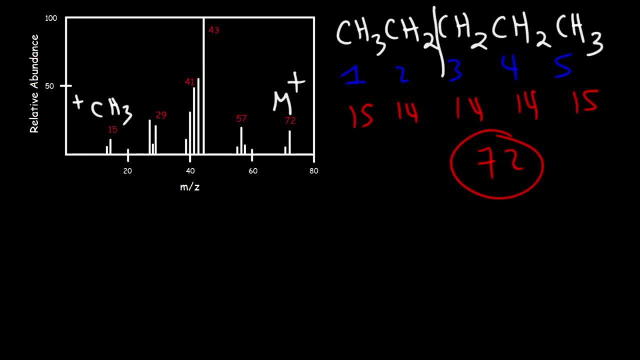 break the C 2, C 3 bond, we can get these two fragments. we can get an ethyl radical or an ethyl cation- but I'm only going to focus on the cations at this point- or we can get a propyl radical or even a propyl cation now, anytime, you see. 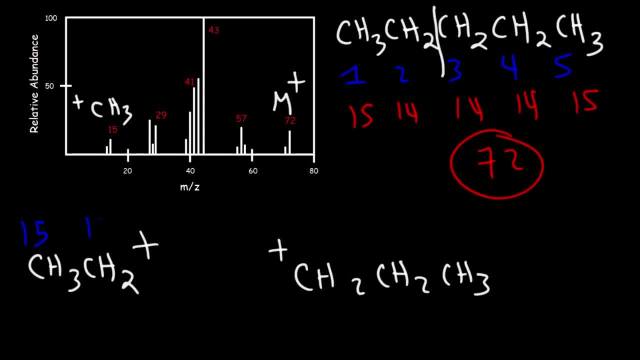 a CH2 group, it has a weight of 15, and a CH2 group has a weight of 14. so the ethyl cation has a weight of 29. so that corresponds to the peak that we see here. as for the propyl cation, if you add 14, 14 and 15, that will give you. 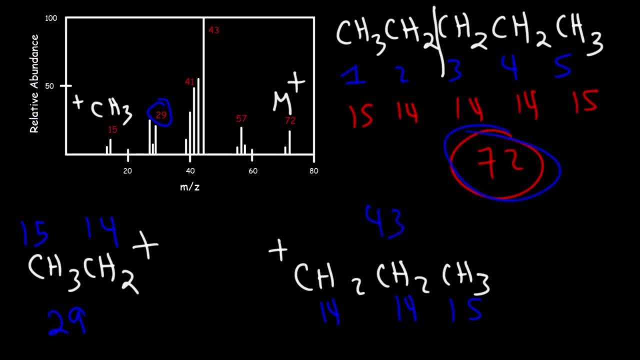 a total of 43, or you could do 72 minus 29 and that'll give you 43. so the propyl cation corresponds to the base peak. now here's a question for you: why is the propyl cation the base peak and not the butyl cation? let's compare both of them. 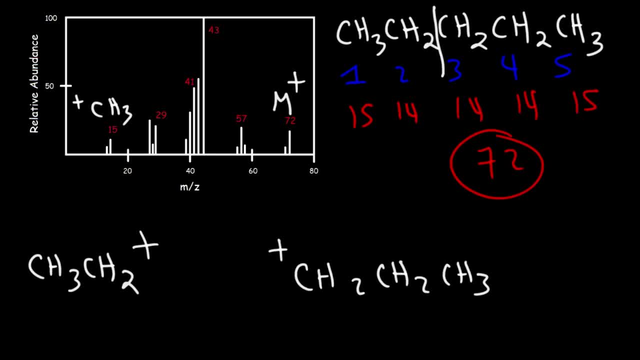 side by side. if we break the C 1- C 2 bond, we could get a methyl cation and we could get a primary butyl cation now, which situation leads to the formation of more stable fragments. in the first scenario where we break the C 2, C 3 bond, notice that we have. 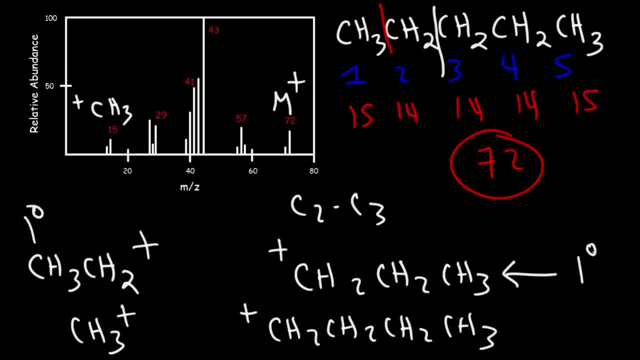 a primary ethyl cation and a primary propyl cation. in the second situation, where we break the C 1- C 2 bond, we have a primary butyl cation and a methyl carbocation. so a methyl carbocation is less stable than a. 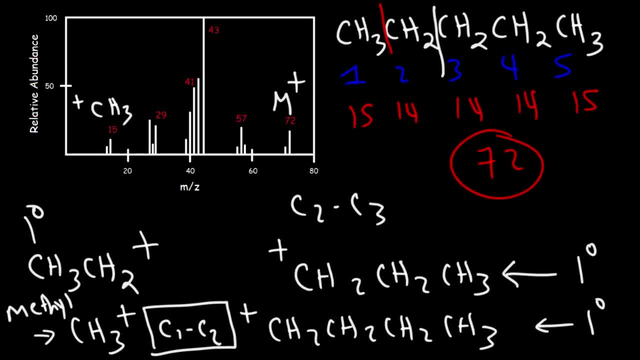 primary carbocation, which means it's easier to break the C 2- C 3 bond as opposed to the C 1- C 2 bond, because this will give us more stable fragments and that's why this is more abundant, because it's easier to break the C 2- C 3 bond. 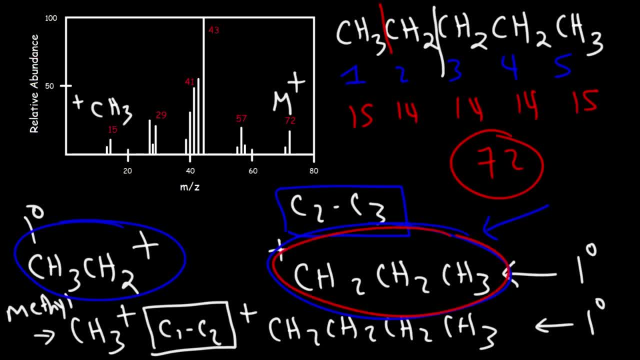 now it's important to understand that both of these cations can rearrange to a more stable secondary carbocation. but the reason why this is the base peak is because it's easier to break the C 2, C 3 bond due to the formation of 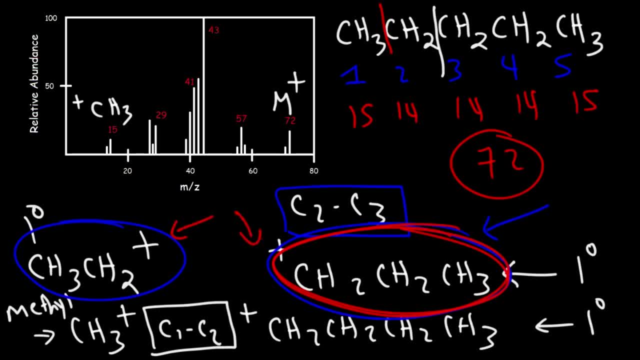 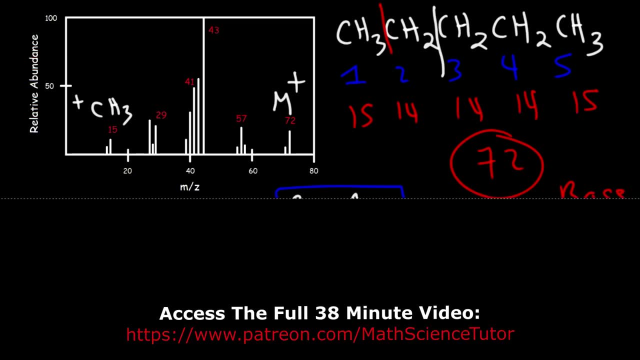 more stable carbocation fragments. this one is less stable, so it's going to be harder to form, and so that's why this corresponds to the base peak. now let's clear away some of the stuff that we have on the board. so at this point we've 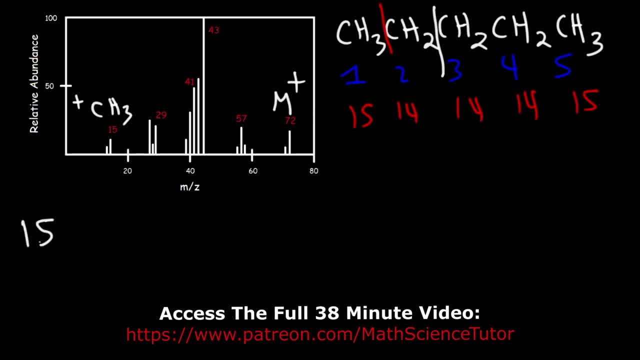 identified all the peaks. so the peak at 15 corresponds to the methyl cation, the peak at 29 corresponds to the ethyl cation, the peak at 43 corresponds to the propyl cation and the peak at 57 corresponds to the butyl cation. at 72. 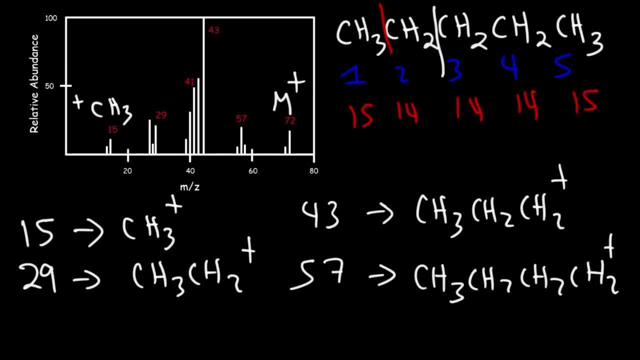 it's the original compound that lost only one electron. now, what about the peak at 41? how can we get that? so, starting with the propyl cation, and this molecule can lose two hydrogen radicals, and if it does so, what's going to happen is we're going to get an allylic carbocation. 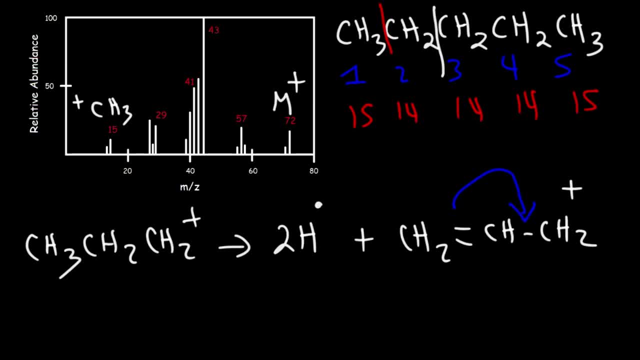 and this carbocation is stabilized by resonance, and so that's why it's very abundant as well relative to the other fragments. so it's relatively easy to form this particular carbocation, its primary and its allylic. so if this has a mass to charge ratio of 43, and if we subtract two from that, then the mass of